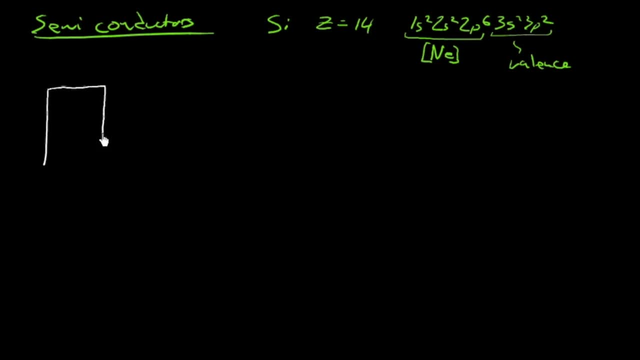 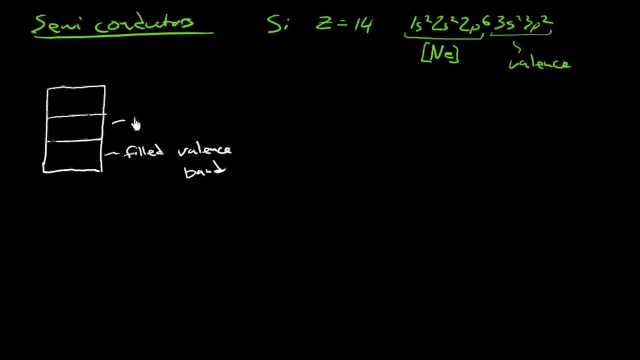 OK, OK, OK, And we have this band gap, We've got this valence band And we have a conduction band And in order to get conduction we need to promote an electron from the valence band across the band gap into the conduction band. 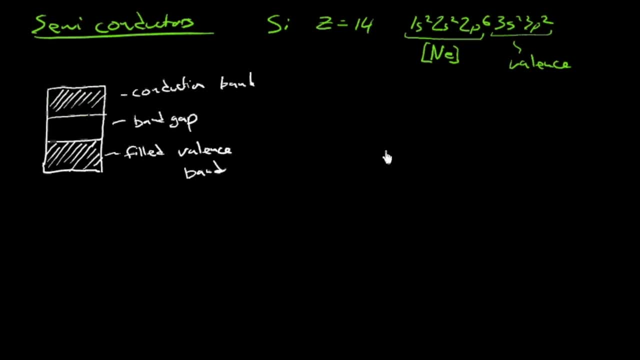 All right, Great, OK, so that's a good look at the band structure. What about if we look at a cartoon sketch of the crystal? I think it'll be a little bit easier perhaps to visualize. But we'll show the same event: that promotion of an electron. 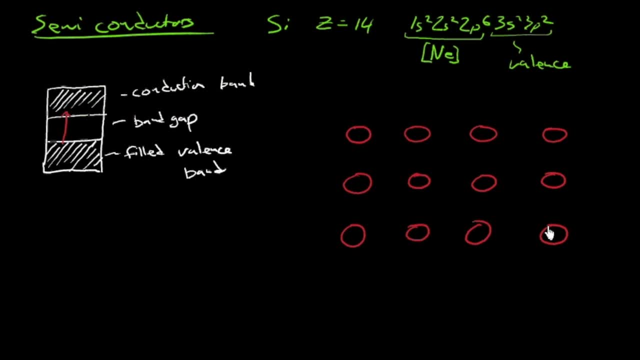 up like this to give conductivity. And so if this is silicon here, each of these little circles is meant to be silicon, And each silicon brings to the table those four valence electrons. So it's going to have four valence electrons like this: 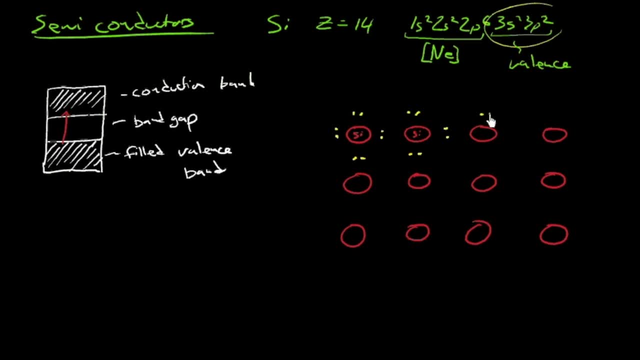 And, of course, it shares those covalently with the adjacent silicons And we get something that we could sketch like this. I mean, this is a two-dimensional representation, of course, But not bad. I mean, this is good enough for our purposes. 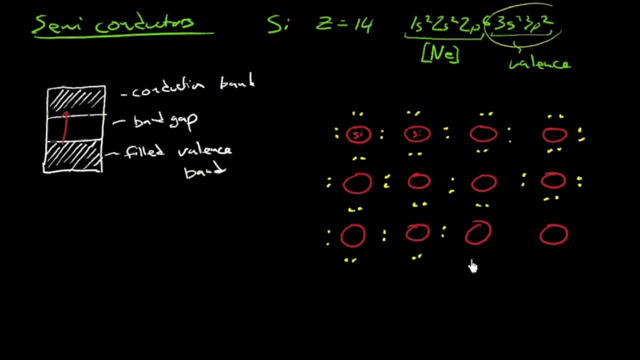 And this is what we're talking about, just these sp3 hybridized electrons. That's kind of what it looks like. I mean, it's again two dimensions, But it's good for our purposes. And so then what happens is when we promote an electron, 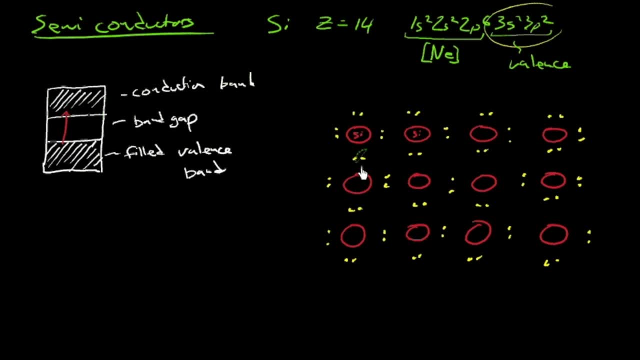 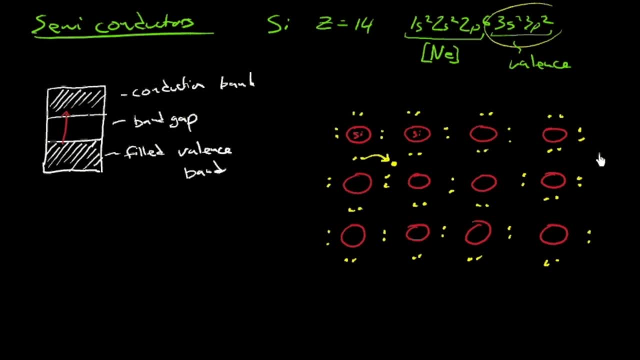 or in the model that we had from the sea of electrons in a metal. We're moving that electron into the conduction band, where it's free of nuclei, So it's left behind a missing electron. OK, so this missing electron is in a place. 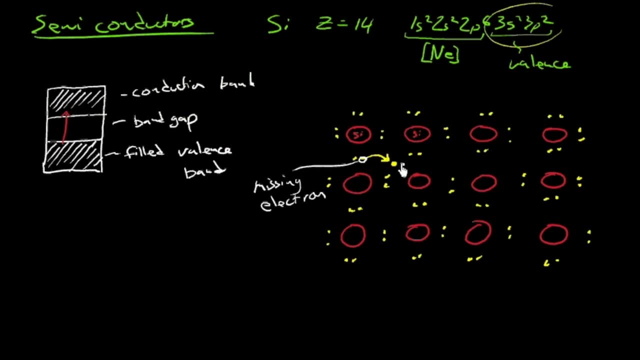 where there would have been a negatively charged electron. Now, remember, this electron is negatively charged, So this is the absence of an electron, the absence of something you could call a hole, And in fact that's often what we do: call this a hole. 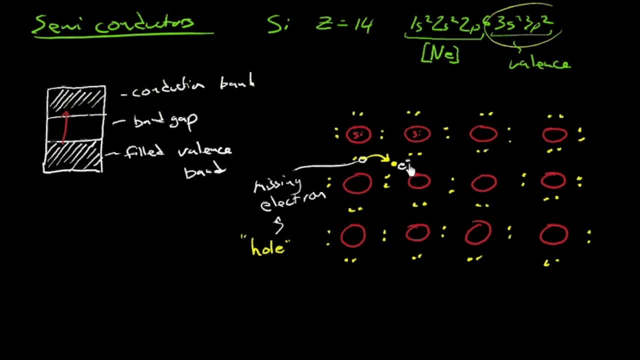 And so the interesting thing is, We've promoted an electron up into conduction. It's free to move, So now it can conduct through this semiconductor. In fact, this model's not bad. You can see this electron moving. It might hit a nuclei. 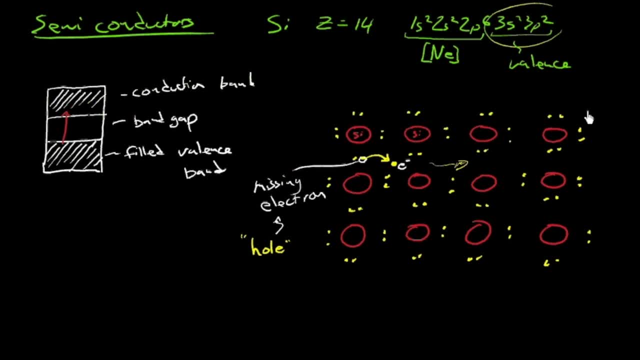 It might get some thermal vibrations there. There could be a grain band or any kind of scattering event that would interfere with the conductivity of that electron. But if the electron's moving this way, say towards a positive electrode, well the hole which is 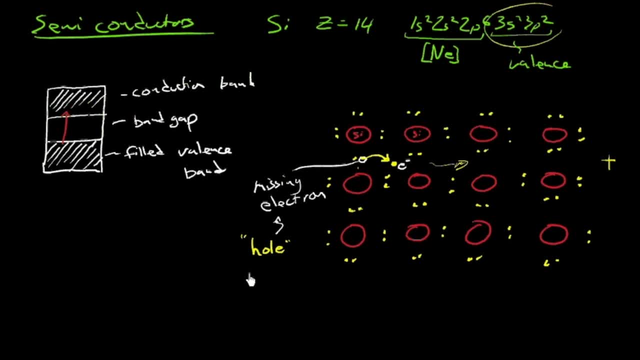 The hole appears to be positive. It appears as if it's positive, And it's a little bit bizarre to think about this hole as being something that you might see moving, But we could, with a little stretch of our imagination, imagine that that hole is something that's moving. 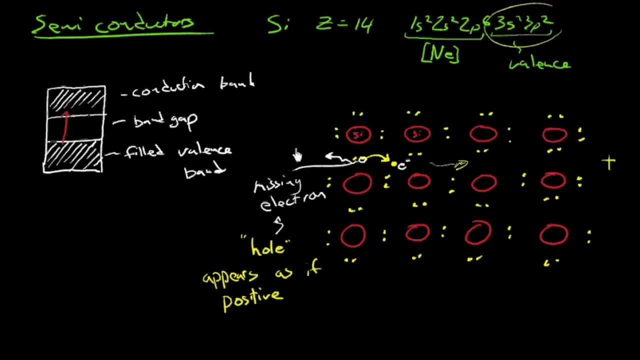 So it's as if the hole is moving, And the other way, say towards the negative electrode. And so we get actually two, we call them charge carriers, Two things that are carrying charge. This is carrying a positive charge And this is carrying a negative charge. 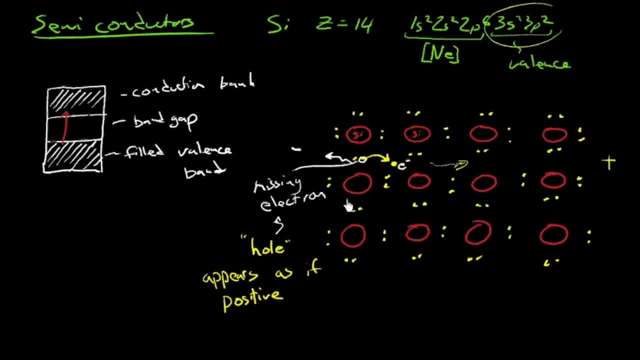 The electron's carrying a negative charge. So there's actually in this example here, where we've promoted an electron up and left behind a hole, We actually have two charge carriers. we say There's two charge carriers And this is actually called intrinsic semiconduction. 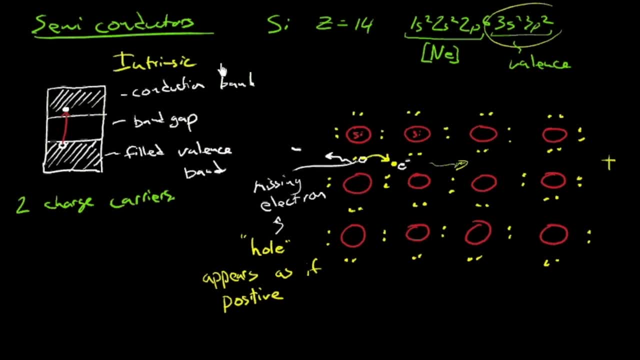 Intrinsic, Intrinsic, semiconduction. And it's intrinsic because this is just the properties of the silicon on its own. We have its own electron promoted up. There's nothing external to this, It's all internal, or we say intrinsic to this material. 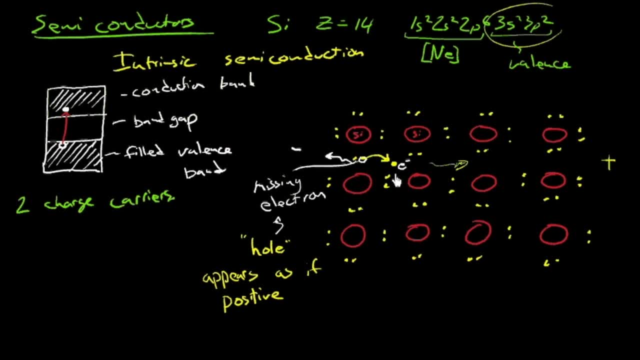 And I'll differentiate that from what we'll cover in a moment where we add some other impurities to this and we dope it. it's called, But right now this is intrinsic semiconduction, It's just the behavior of the material, in this case silicon. 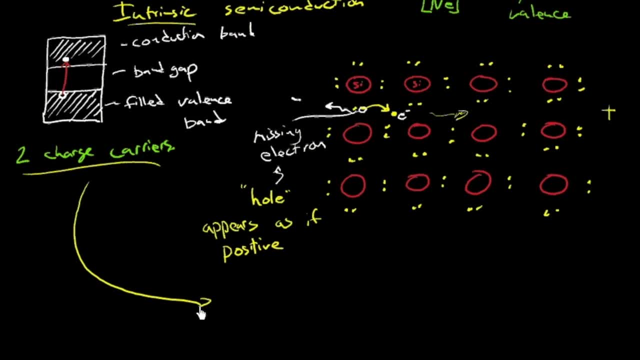 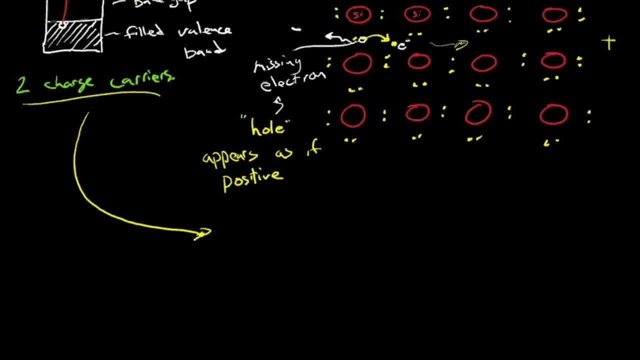 on its own. It's got two charge carriers. So, in fact, the conductivity, if we were to calculate it, it's going to be the same. If we were to calculate the conductivity, it would have to be calculated in terms of the two charge carriers. 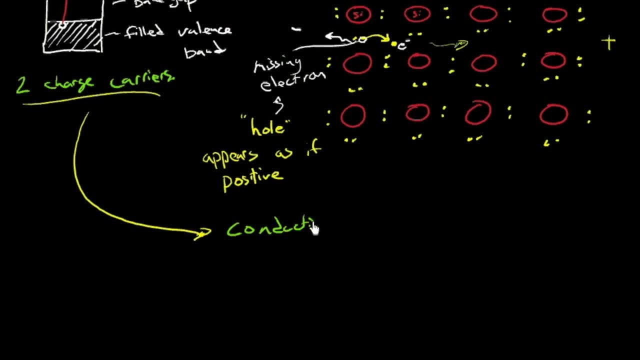 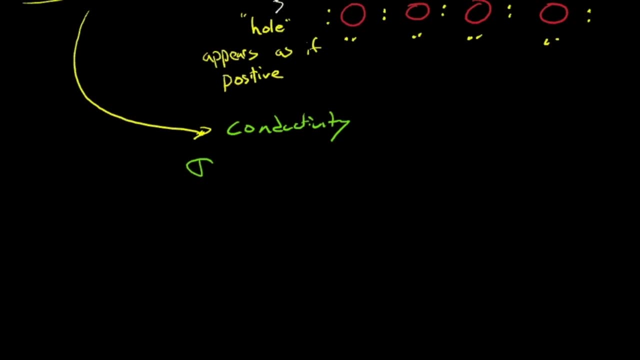 And the conductivity is given the symbol sigma And it's going to be, you can kind of imagine it should be a function of the number of electrons, Times whatever charge that electron is carrying, And I'm giving it the absolute value of the charge here. 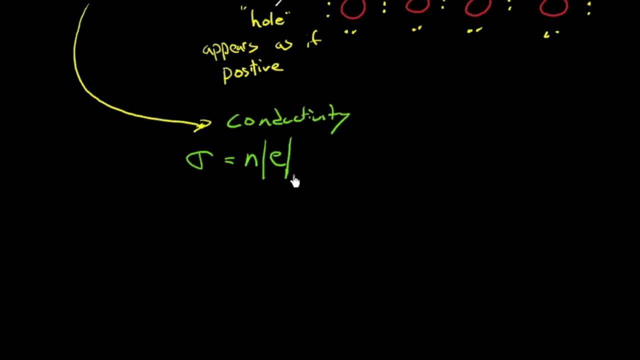 Times how easily the electron can move, And so we have this symbol here for the. this is new sub e for the mobility of the electron. So how quickly is the electron moving, What charge is it carrying, And how many are there? 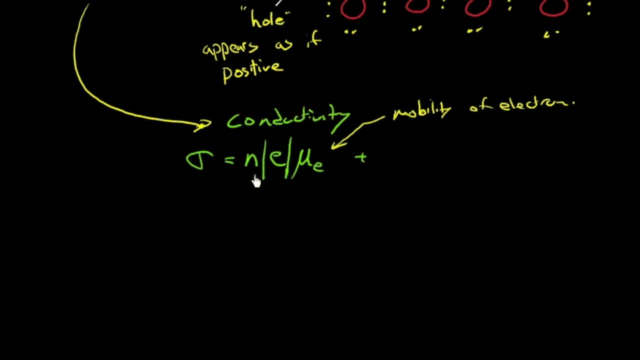 But that's only for the electron. We need to also consider- you could say that's n sub e- We also need to consider the number of these holes, or the positive charges, In fact, actually, you know what. sorry, let me clear it. 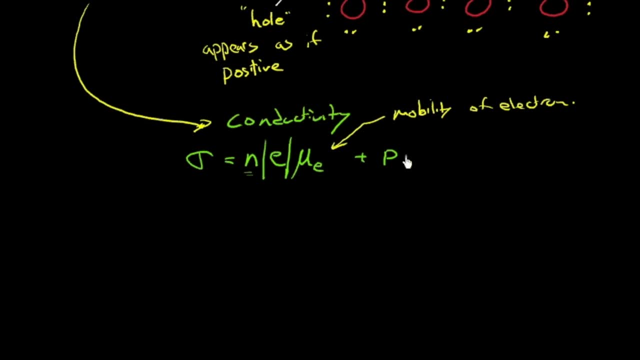 I'm going to leave this n for negative And we're going to put p for positive. So that would be the number of positive charge carriers Times their charge But they're carrying just. the absolute value of their charge is the same And then times the mobility of those charge carriers. 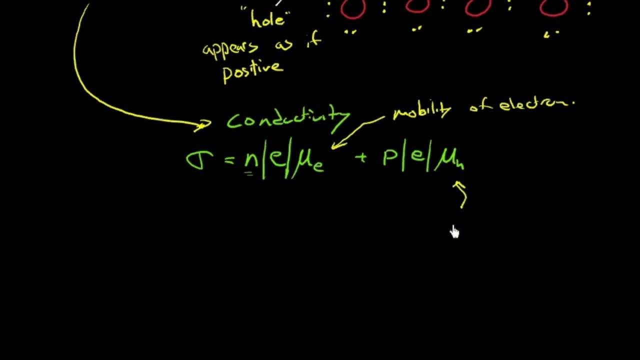 And I put subscript h because these are holes. So that's the mobility of a hole And p is the number of holes And of course Number of electrons promoted is going to be actually the same as the number of holes. So we could actually simplify this equation. 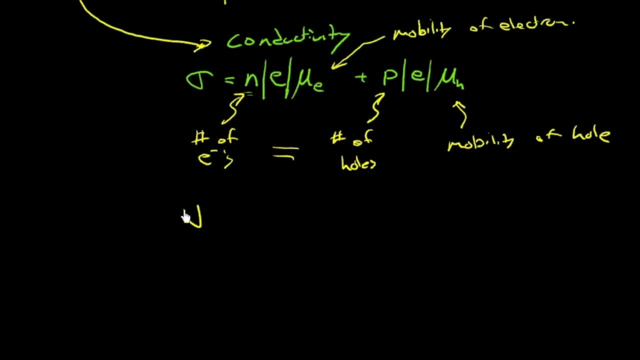 Which I'll do. Simplify this. We could say that the conductivity of an intrinsic semiconductor is going to be equal to the number of intrinsic charge carriers times the fundamental charge, That's the absolute value of the charge on an electron And, at times, the sum of the electron mobility. 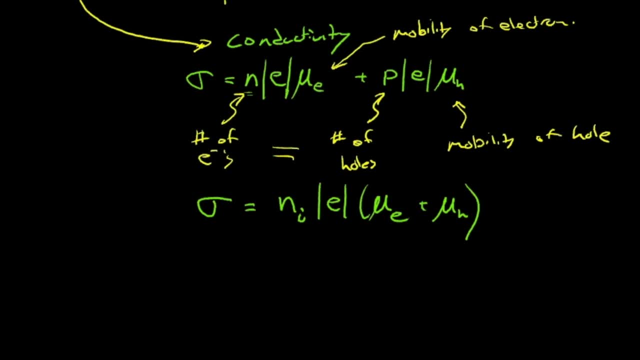 and the hole: mobility. So there we go. That's our equation for the conductivity, And I'll just give you the units here. This is, This is correction, This is: This is number per volume, OK, Per cubic meter. This fundamental charge, of course, has units of coulombs. 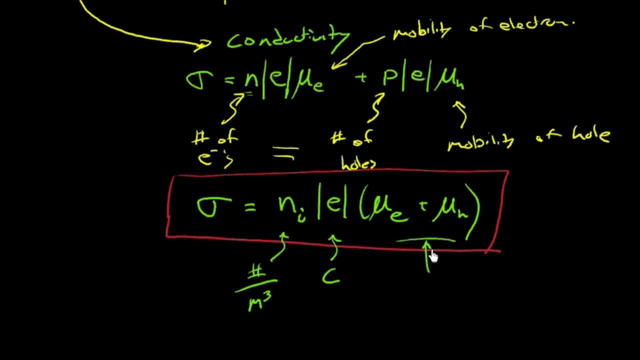 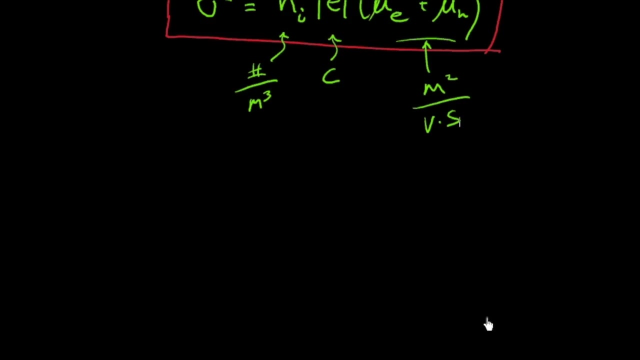 And mobility is going to have units. It's going to have units of meters squared, Meters squared Per volt. Volt Second, And remember, volt is a joule per coulomb. All right, So that's an intrinsic semiconductor. 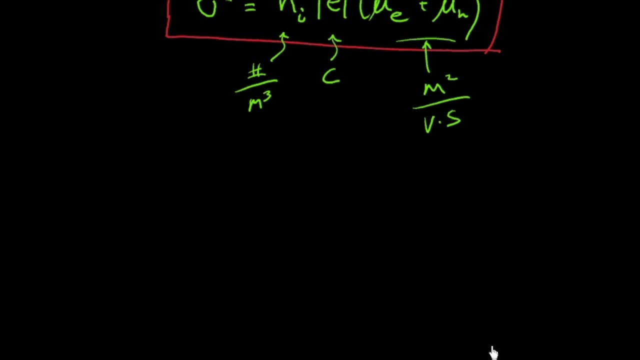 Let's consider, as I hinted, what if we added something to it to change the properties. And so what we're going to do is we're going to make what we call an extrinsic semiconductor. So we need to add something to it so that the properties 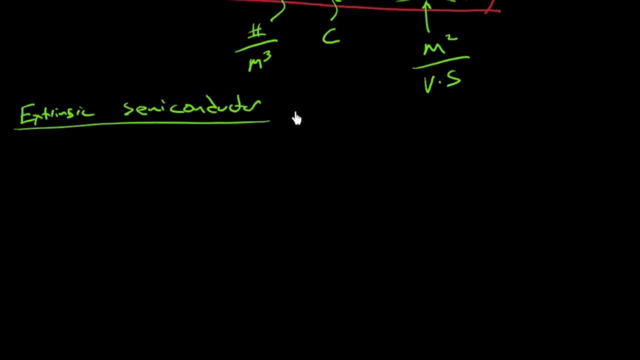 the properties are dominated by that, something that we add in. OK. And so what we're going to do is we're going to say let's add a tiny little amount of something that's got a different number of electrons, So say, we'll add some phosphorus. 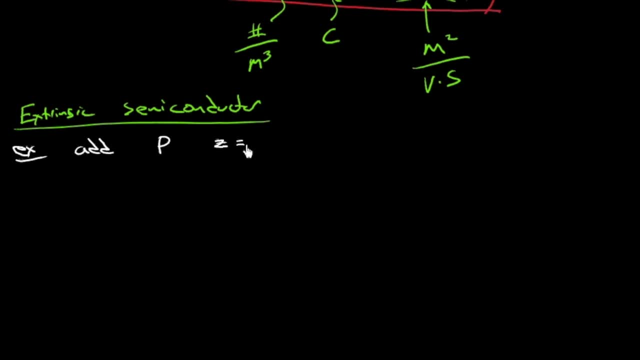 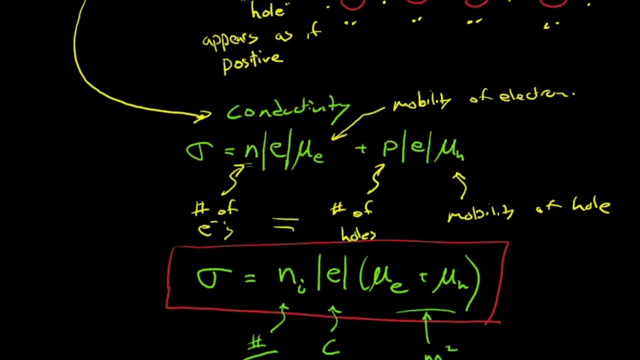 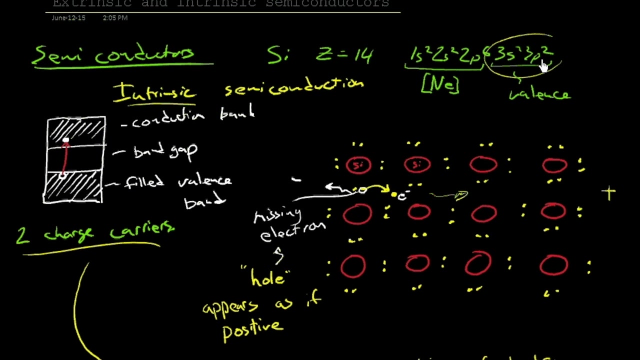 OK, Well, phosphorus has an atomic number or a proton number of 15.. Right, So it's going to have that same electron Electron configuration that we had for silicon right up here: 3s2, 3p2, except plus one extra. 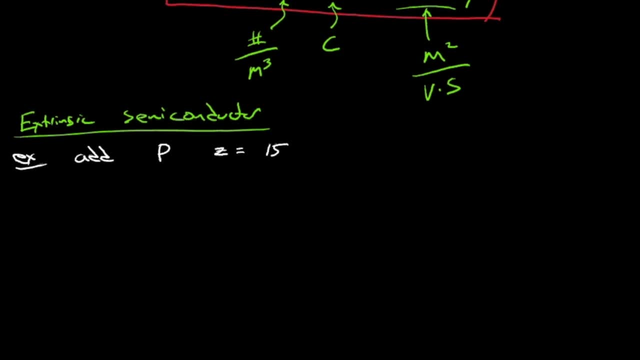 So it's going to be 3s2- 3p3.. All right, So that's going to be neon 3s2- 3p3.. It brings this extra electron, if you will. I mean, it's just an extra because it's in quotes. 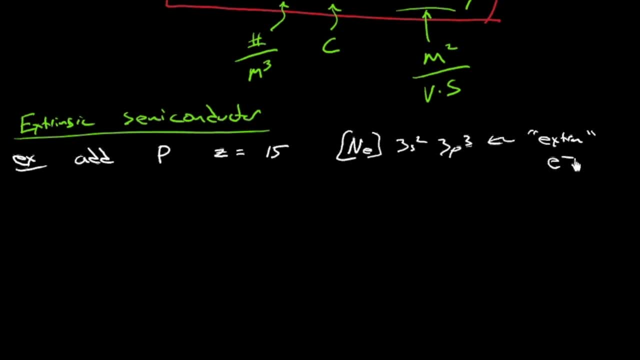 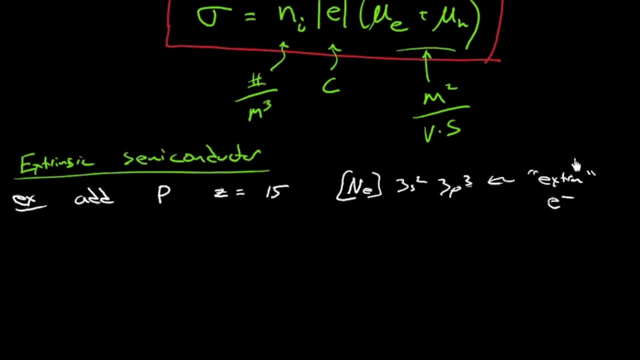 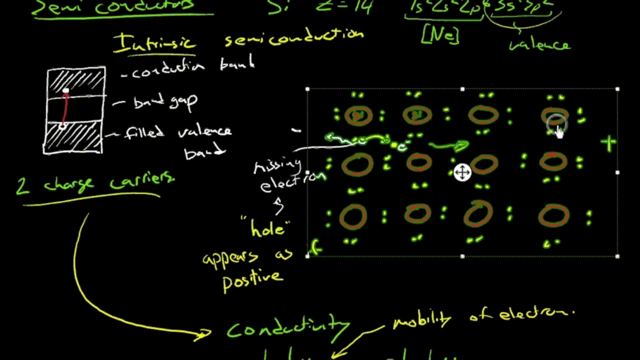 I'm saying extra, It's relative to silicon, But it brings this extra electron to the table, And so what's going to happen is, let's see, I'm going to just copy this for you. OK, I'm going to copy that, bring it down here. 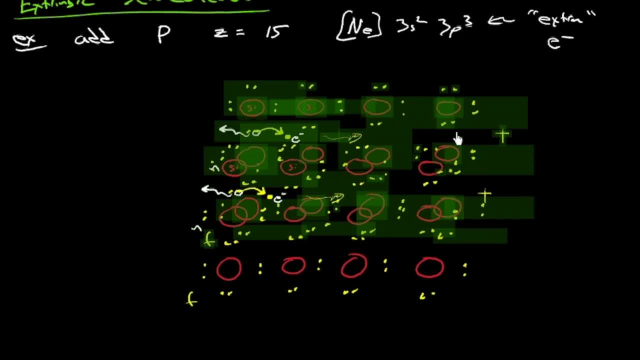 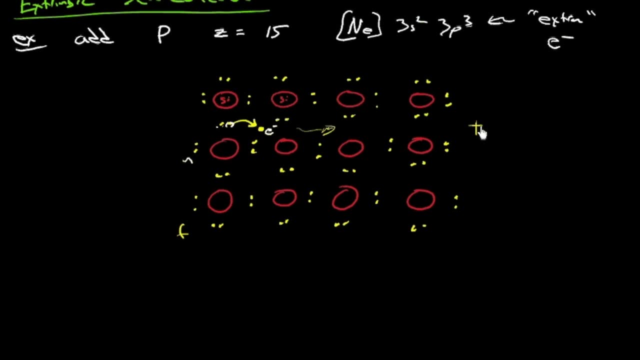 And we can use our- we can start with our- silicon here, And what we're going to do is then we're going to say, OK, Let's actually just replace this one of these. We're going to make a little point: defect here. 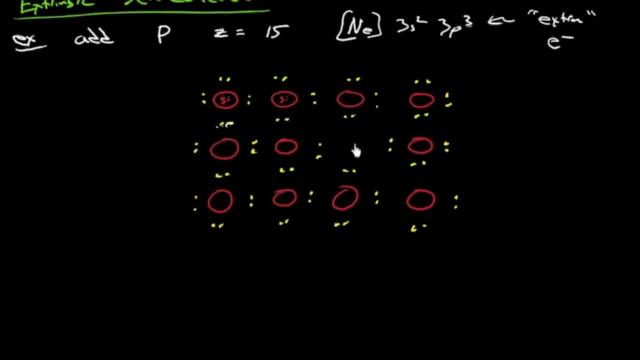 So we're going to actually replace one of these silicons with phosphorus. OK, So not that there's any significance to the color, but I'm going to make that phosphorus. And remember, phosphorus had five valence electrons, So it would have contributed, say, these ones here: 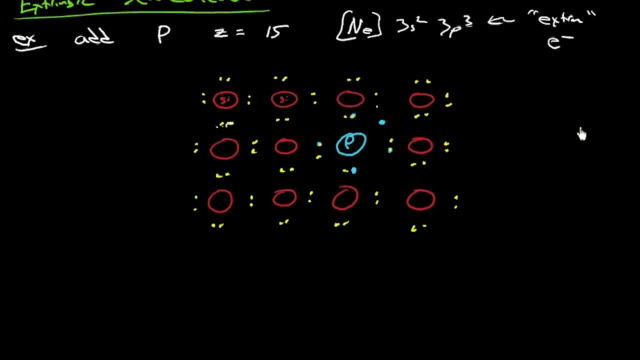 for the bonds. But then it's still got one extra. OK, And that one extra, it's shielded by these core electrons. It's really weakly attracted, It's weakly bound, Or another way of looking at that is in terms of the band diagram. 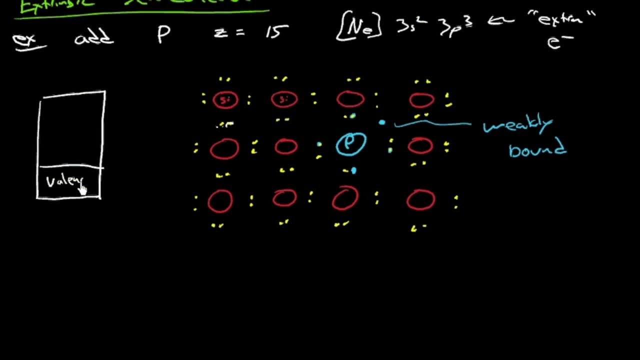 This is the valence band, This is the conduction band. This extra electron really is really close to being free, So it's got an energy that's kind of already pretty close to the conduction band. That is, you need a very small amount of energy. 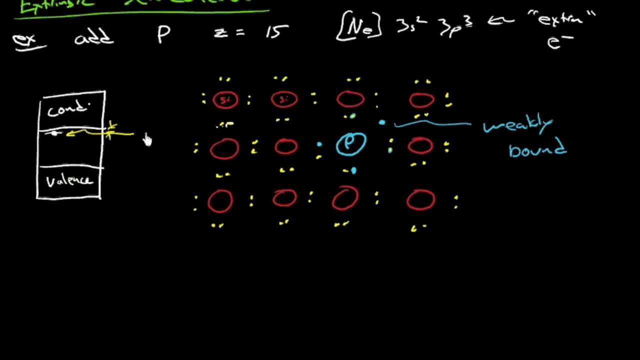 to promote that electron and make it free. And remember what is this? This is phosphorus, donating an electron, So we call that the donor level. That's the donor level, And what's it? Lever? No, no, Not lever. 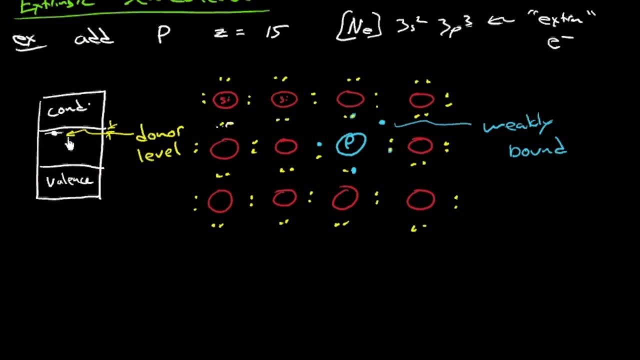 Level: Donor level. That's the donor energy level, because phosphorus is donating an electron And it's very close to the conduction band, So it can quite easily do it. In fact, that means that there's going to be far more of these contributed or donated charge. 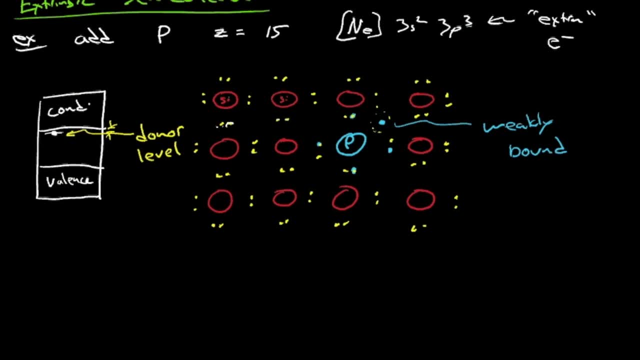 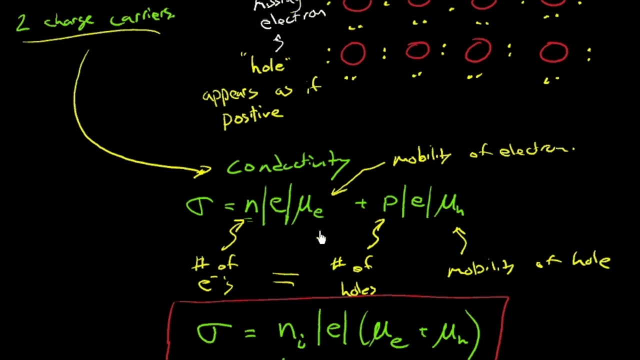 carriers than the intrinsic ones, And so the conductivity, then the extrinsic conductivity. it won't be influenced very much by the intrinsic, Intrinsic, Intrinsic, Intrinsic, Intrinsic Intrinsic Properties, The contributed or donated electrons. 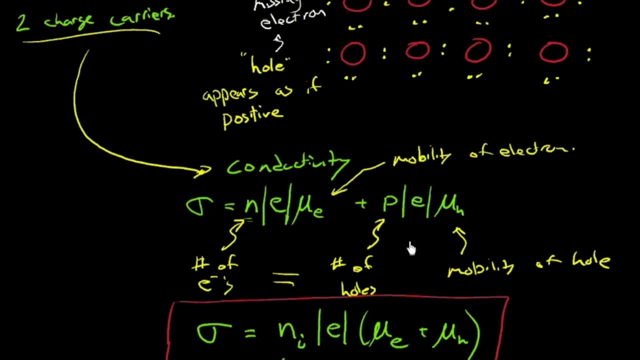 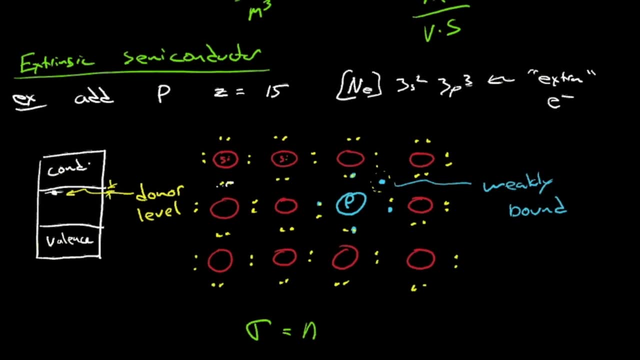 are going to dominate, And so we can actually eliminate the contribution from the holes, because there's very few holes. The holes are just the intrinsically generated holes, But we've got mostly the extrinsically contributed electrons, So our equation for conductivity would just now. 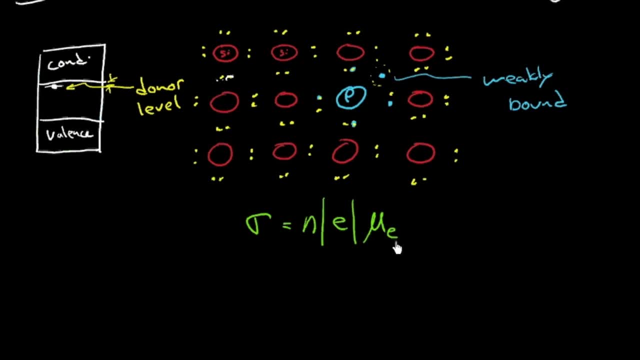 involve the electron mobility, And similarly we could dope with: oh and so actually. so one last thing is: the charge carrier is the electron, And the electron is negative. So we call this an n-type semiconductor, an n-type.